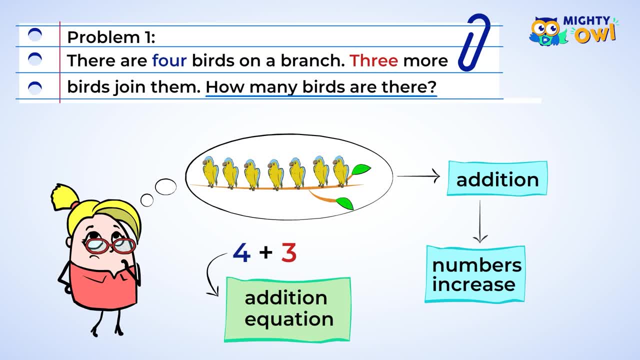 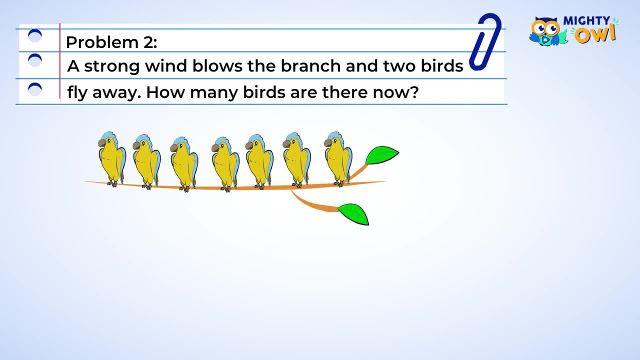 Take a look: Four birds plus three more, Well, there are seven birds on the branch now. Well, what if we continued with this example and said: a strong gust of wind blew the branch and two birds flew away. Now you have two birds leaving. So what you need is the math operation. 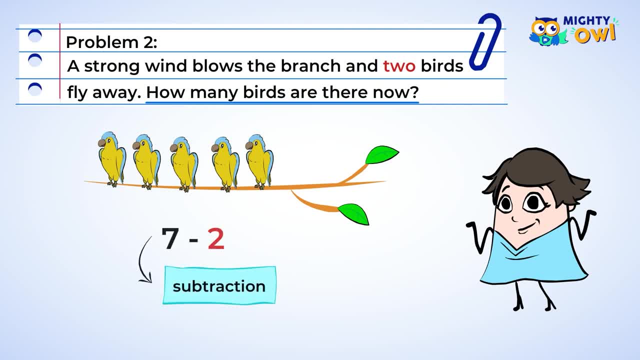 of subtraction. This way, you can show that birds are leaving or that the number of birds are getting smaller. This means we can take seven birds and put them on the branch And subtract two, And now five birds are left on the branch. Okay, that wasn't too hard, was it? 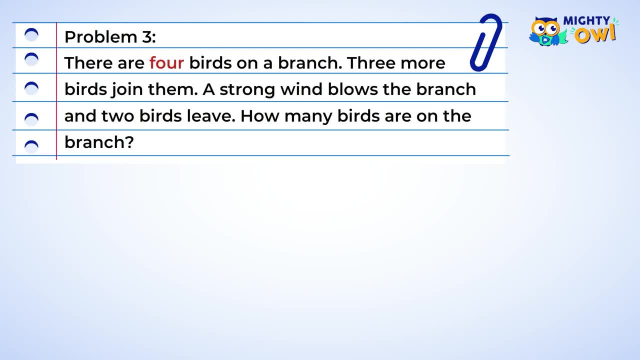 But what if the two problems were combined? Four birds are on a branch, Three more birds join them, A strong gust of wind blows the branch and two birds leave. How many birds are still on the branch? Well, you've actually already solved this. You used addition and subtraction. 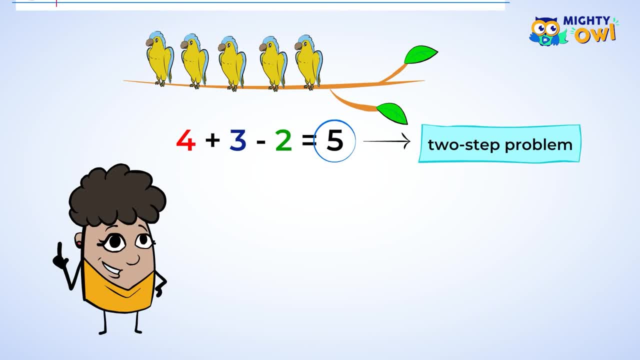 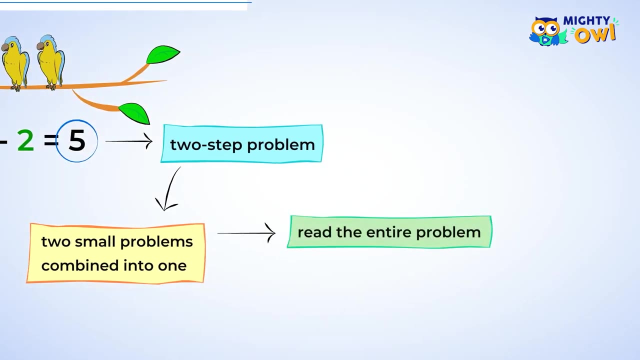 This is called a two-step problem. A two-step problem has two small problems combined into one. Let's go over the different steps to solve two-step problems. First and foremost, we want to read the entire problem. Sometimes problems can be a bit long, So we want to take 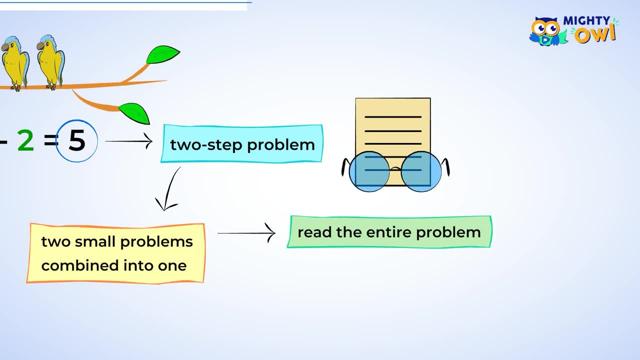 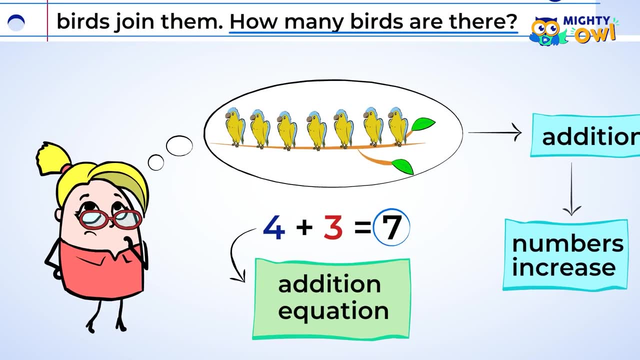 our time and we want to read the whole thing. Next, we want to think about what the problem is asking. It may help to visualize the problem. We want to think about what the problem is asking, Or even make a drawing of what the problem is asking. We can underline the question or. 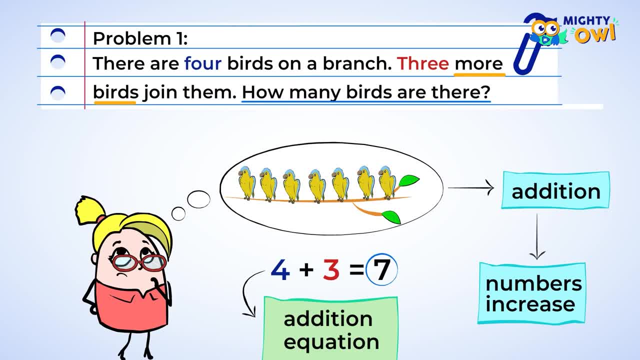 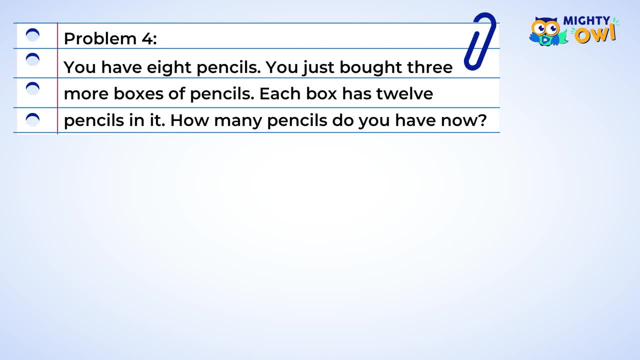 key words, if that helps us, And finally we create an equation to solve it. Let's use these steps to solve an example problem. Here it comes, Okay. first we read the problem. You have eight pencils. You just bought three more boxes of pencils and each box has 12 pencils in it. How many pencils? 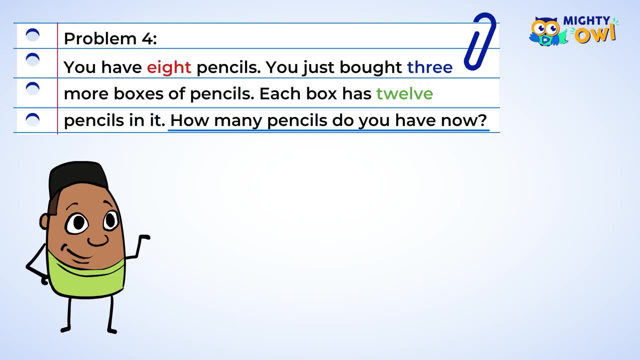 do you have now? Second, let's visualize Picture this: You have eight pencils. You just bought three boxes. Now, buying indicates addition, So we're going to be adding more pencils. We know that each box has 12 pencils. Huh, this sounds like equal groups, Three groups of 12.. Right, 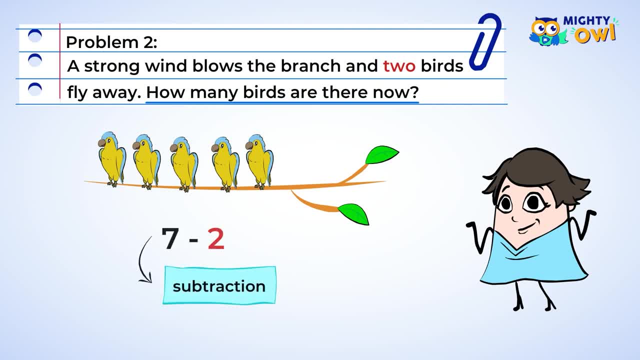 of subtraction. This way, you can show that birds are leaving or that the number of birds are getting smaller. This means we can take seven birds and put them on the branch And subtract two, And now five birds are left on the branch. Okay, that wasn't too hard, was it? 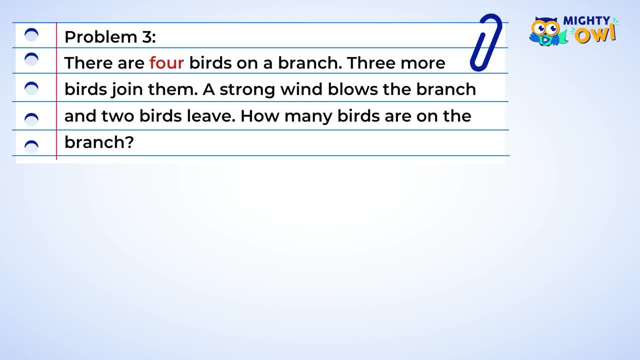 But what if the two problems were combined? Four birds are on a branch, Three more birds join them, A strong gust of wind blows the branch and two birds leave. How many birds are still on the branch? Well, you've actually already solved this. You used addition and subtraction. 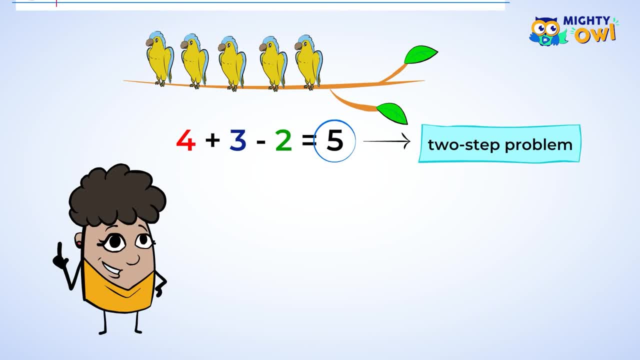 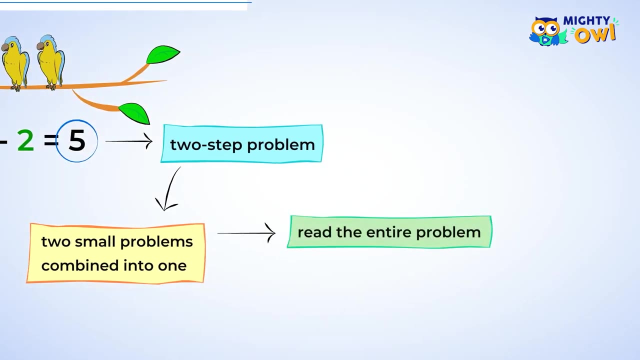 This is called a two-step problem. A two-step problem has two small problems combined into one. Let's go over the different steps to solve two-step problems. First and foremost, we want to read the entire problem. Sometimes problems can be a bit long, So we want to take 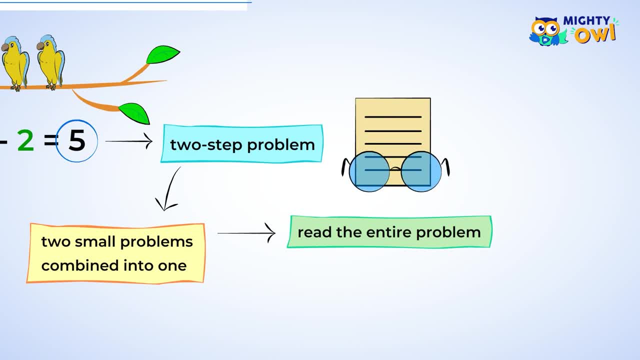 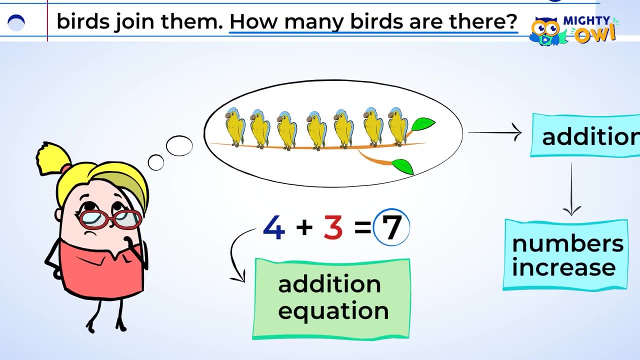 our time and we want to read the whole thing. Next, we want to think about what the problem is asking. It may help to visualize the problem. We want to think about what the problem is asking, Or even make a drawing of what the problem is asking. We can underline the question or. 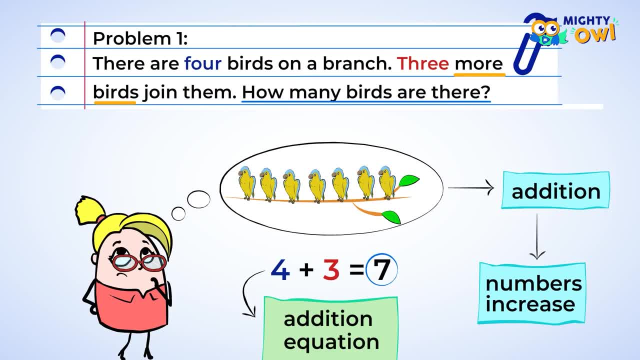 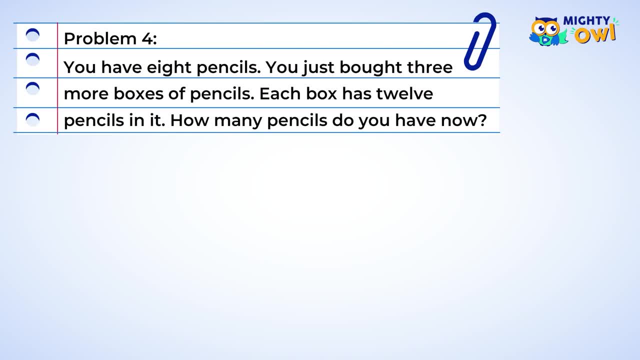 key words, if that helps us, And finally we create an equation to solve it. Let's use these steps to solve an example problem. Here it comes, Okay. first we read the problem. You have eight pencils. You just bought three more boxes of pencils and each box has 12 pencils in it. How many pencils? 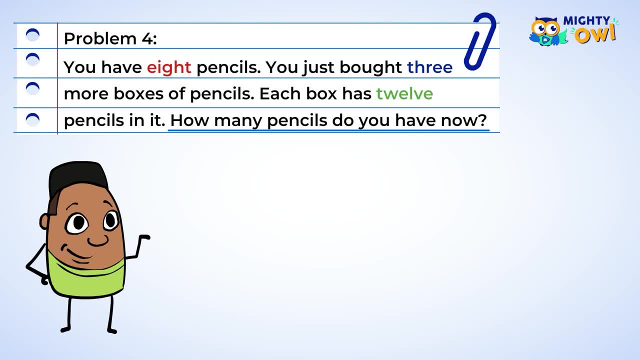 do you have now? Second, let's visualize Picture this: You have eight pencils. You just bought three boxes. Now, buying indicates addition, So we're going to be adding more pencils. We know that each box has 12 pencils. Huh, this sounds like equal groups, Three groups of 12.. Right, 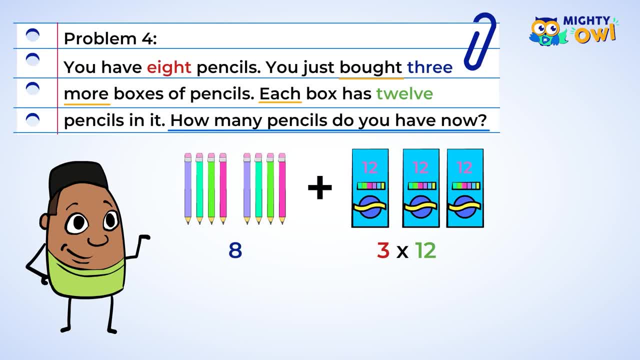 that is multiplication: Three multiplied by 12.. Looks like you have the equation to solve: Eight plus the product of three times 12.. Let's start with the new pencils you just bought. Three times 12 is 36.. So you bought 36 new pencils, Okay. 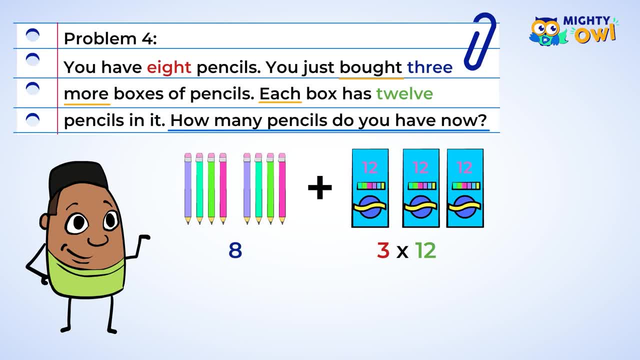 that is multiplication: Three multiplied by 12.. Looks like you have the equation to solve: Eight plus the product of three times 12.. Let's start with the new pencils you just bought. Three times 12 is 36.. So you bought 36 new pencils, Okay. 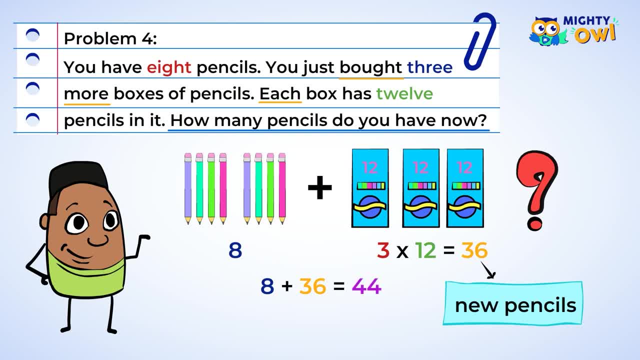 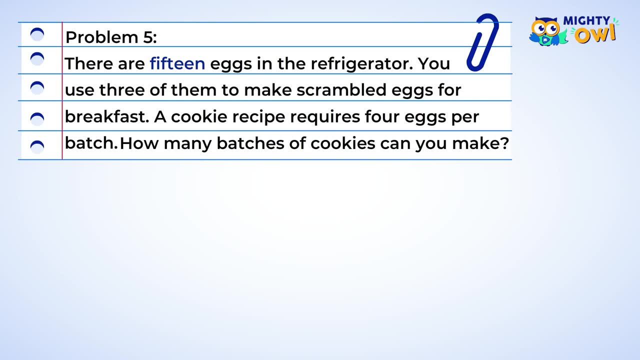 eight plus 36 is 44. So you now have 44 pencils altogether, And you are well supplied to do even more math practice. Let's look at one of those new pencils, because here comes another problem. There are 15 eggs in. 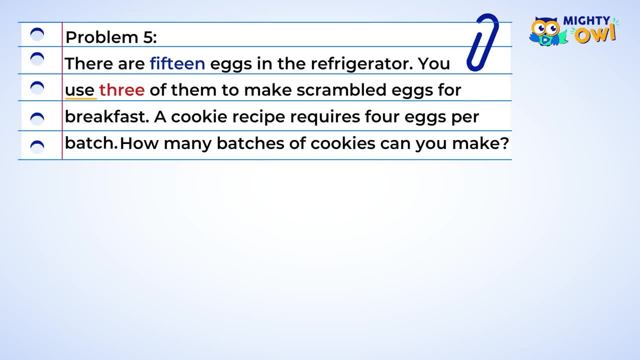 the refrigerator. You use three of them to make scrambled eggs for breakfast, And a cookie recipe requires four eggs per batch. So how many batches of cookies can you make? Well, let's look at the situation, Remember. first, we want to identify what the problem is asking. There are eggs, but you ate. 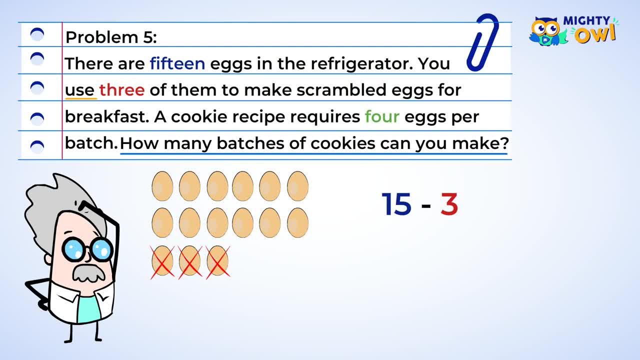 two, So we can make five boxes of cookies. andffer your answer, So that makes up for the biggest amount of eggs broken. What else Two? We think it's a pretty fancy explanation. It's fine if we're right on. There is a weird thing that happens when it turns into a quiz game. 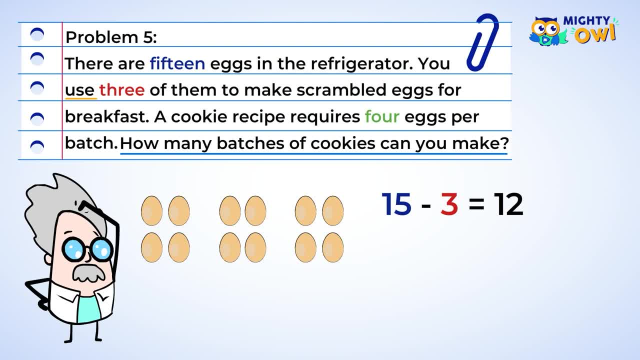 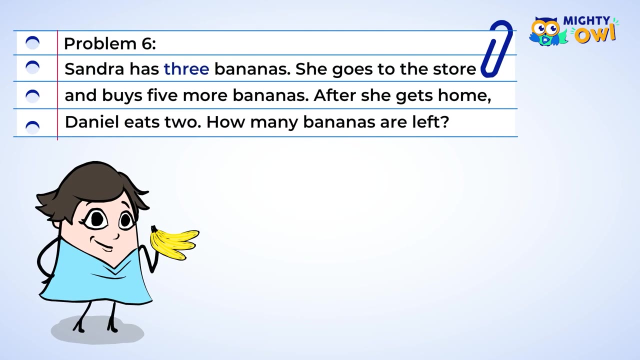 The main thing to think about is that in something simple and easier than this, the most basic is three, So you can make three batches of cookies. Let's try another problem. Sandra has three bananas. She goes to the store and she buys five more bananas After she gets. 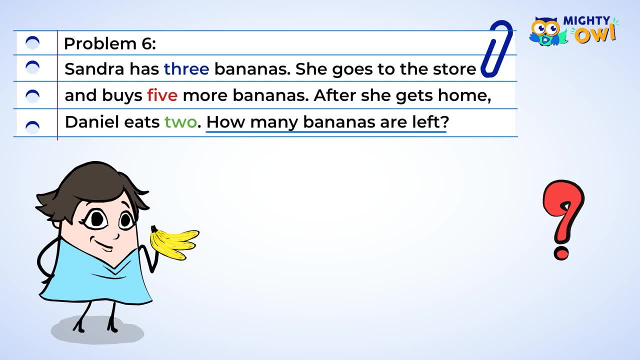 home, though, Daniel eats two. How many bananas are left Now when Sandra goes to the store and buys more? that means that she is adding more bananas, And this means you want to start by adding three and five. Three plus five equals eight. Next, Daniel eats some bananas. This means 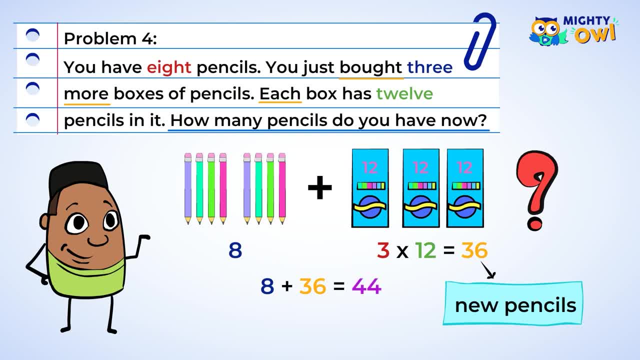 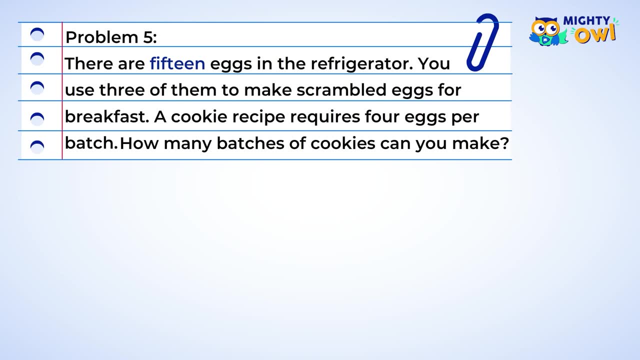 eight plus 36 is 44. So you now have 44 pencils altogether, And you are well supplied to do even more math practice. Let's look at one of those new pencils, because here comes another problem. There are 15 eggs in. 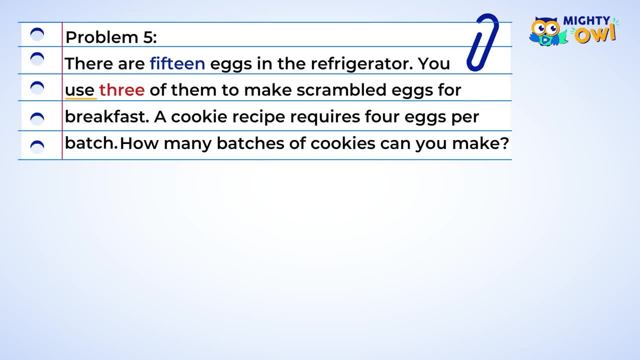 the refrigerator. You use three of them to make scrambled eggs for breakfast, And a cookie recipe requires four eggs per batch. So how many batches of cookies can you make? Well, let's look at the situation, Remember. first, we want to identify what the problem is asking. There are eggs, but you ate. 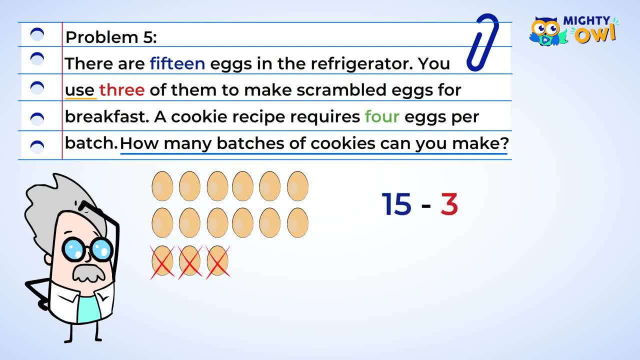 some, And that would indicate Subtraction, since they were taken away: 15, we subtract three, That's 12.. Next, you want to use some eggs for your batches of cookies. We know that each batch has four eggs in it, So we group. 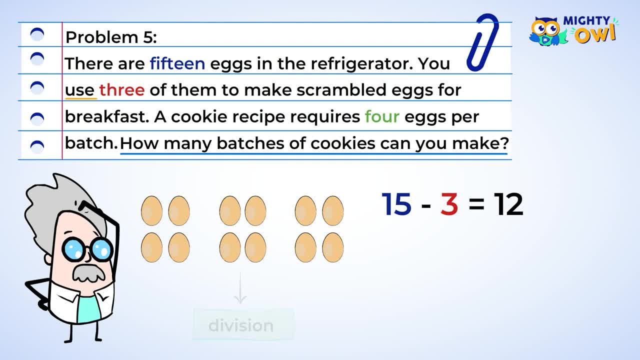 them by four. Okay, putting objects into groups is division, And when we put them into groups of four, there are three groups, Because 12 divided by four is three. So you can make three batches of cookies. Let's try another problem Sandra has. 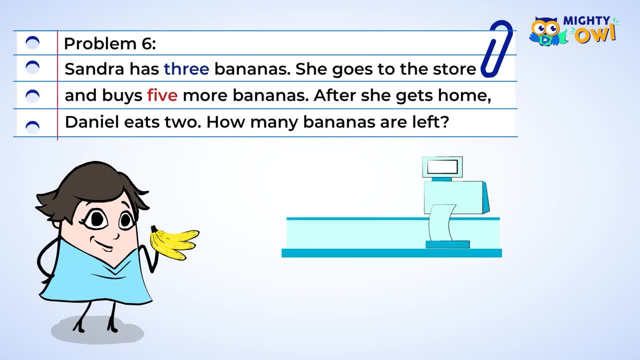 three bananas. She goes to the store and she buys five more bananas After she gets home, though Daniel eats two. How many bananas are left Now when Sandra goes to the store and buys more? that means that she is adding more bananas, And this means you want to start by adding three. 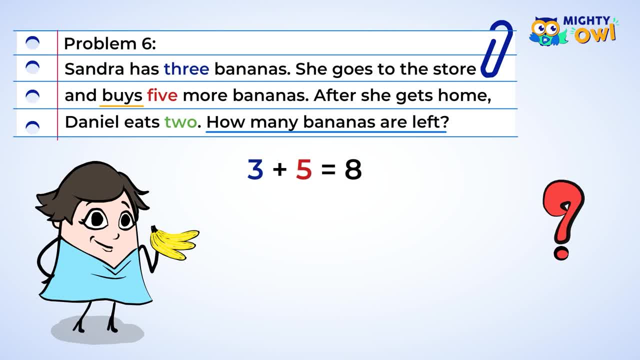 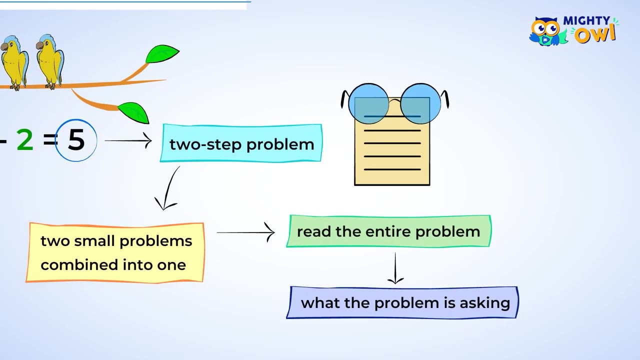 and five Plus five equals eight. Next, Daniel eats some bananas. This means that you'll need to use subtraction Eight minus two is six, So there's six bananas left. Woo, I think you deserve a banana split to celebrate. Now let's go over all that you learned today. Two-step problems are like: 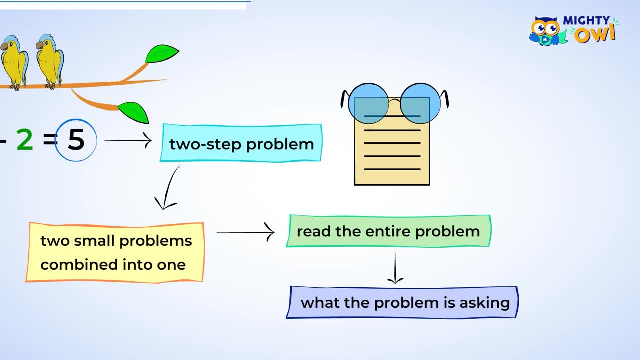 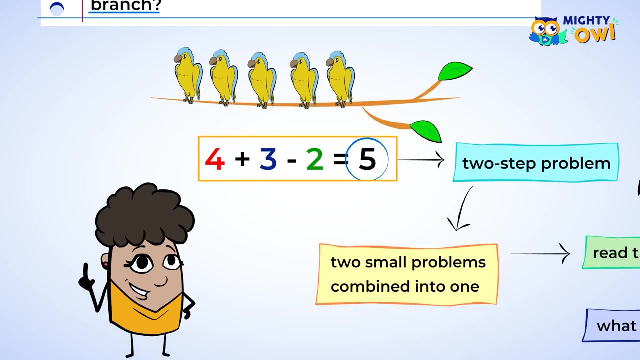 two small problems combined into one. In order to solve, we need to first read the whole problem very carefully And then, second, we need to understand what is being asked and to visualize it, And finally we create an equation to solve it. Great work with problem. 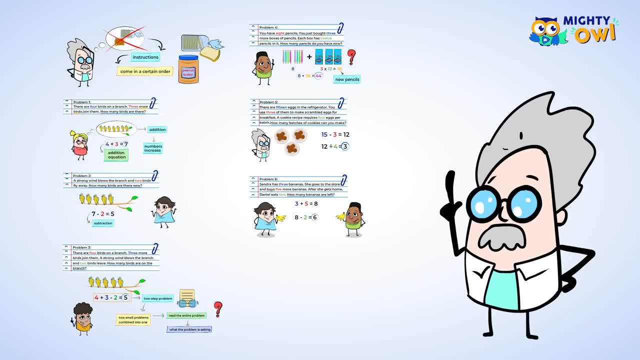 solving, You are becoming a math master.